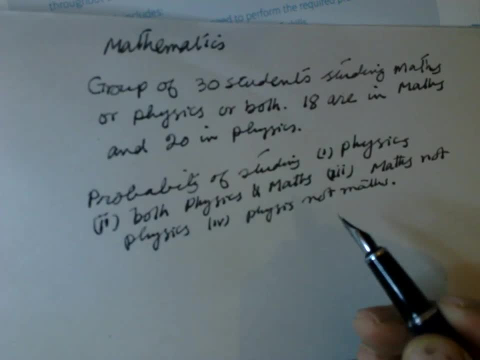 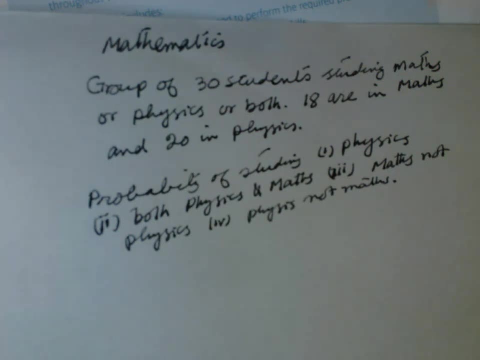 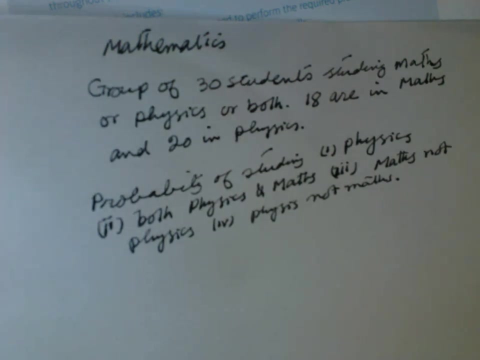 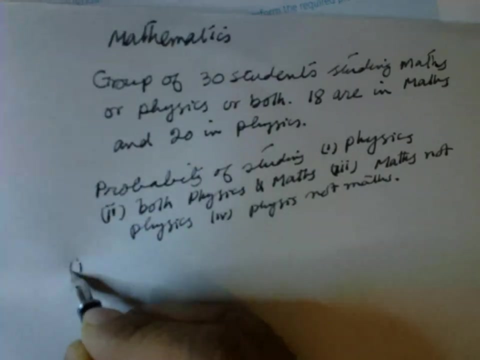 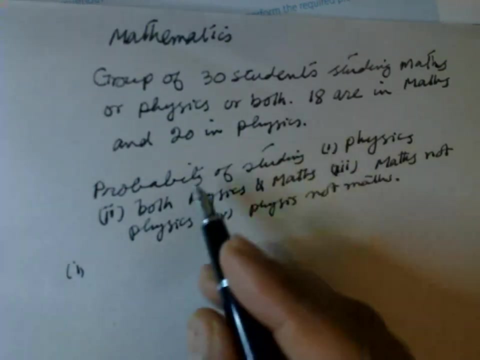 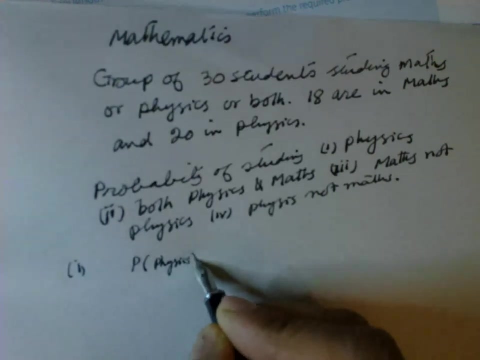 Mathematics. So this is a question: The group of 30 students studying mathematics or physics or both. 18 students are in maths and 20 in physics. Then we have to find the probability of the students studying in physics, So the probability of the physics one is 20.. Probability of physics students is equal to 20 out of 30.. So which is equal to 2 by 3 by 2.. 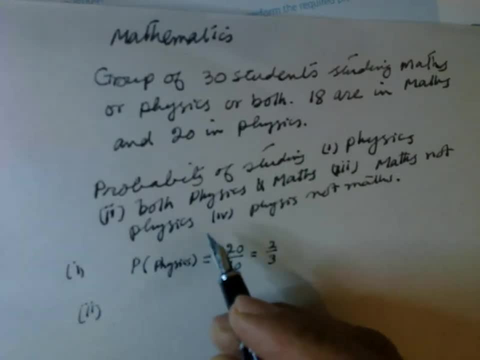 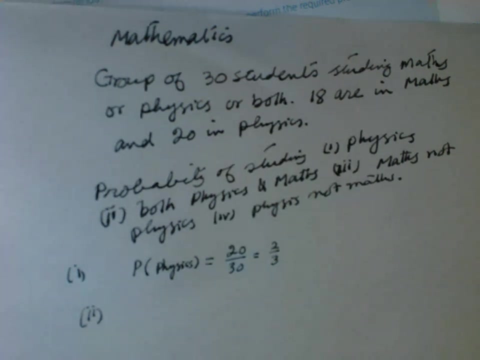 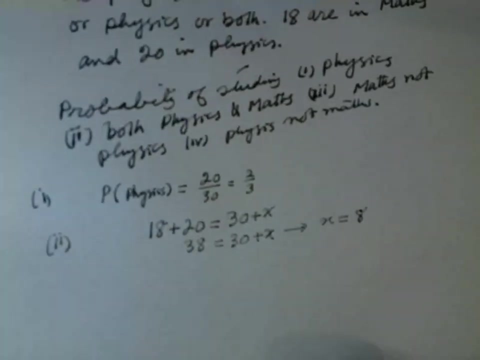 The probability of both Physics. So in this case. so we have to find: 18 are in mathematics plus 20 in physics, which is equal to total plus x. So 38 is equal to 30 plus x. That means x is equal to 8.. So 8 students are studying both. 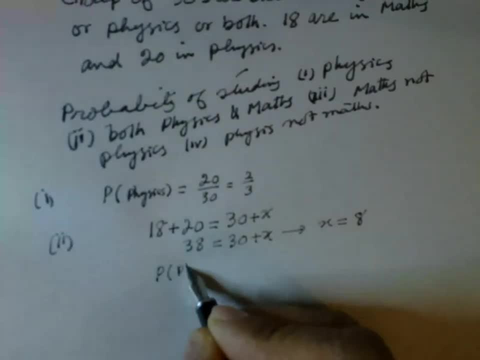 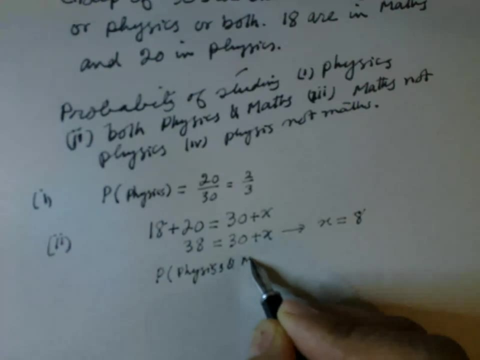 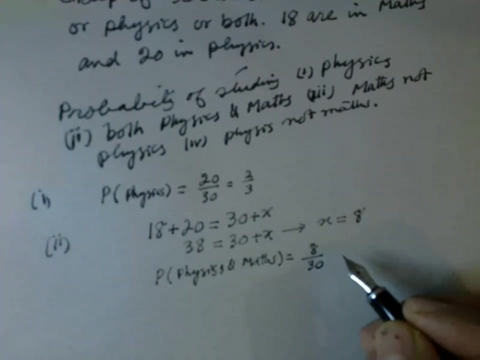 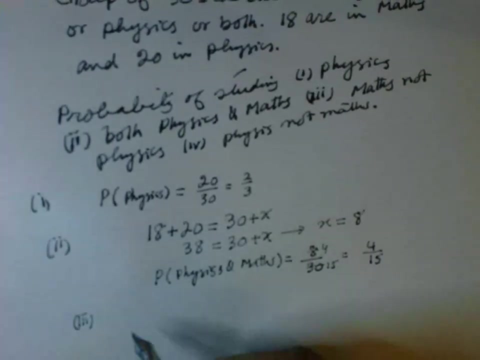 So probability of physics and maths- Math is equal to 8 over 30.. So that will be equal to 4 over 50.. Number 3. Math, not physics. So number of students in mathematics are 18.. So both are 8.. So that is 10.. 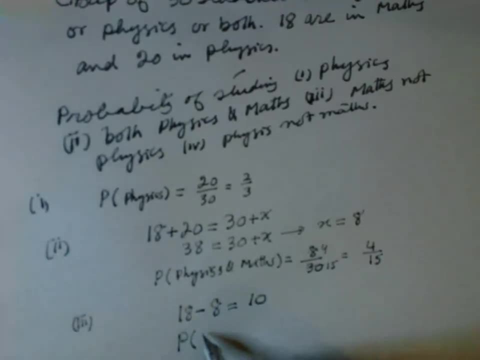 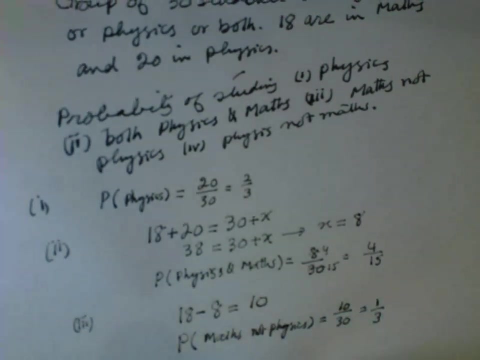 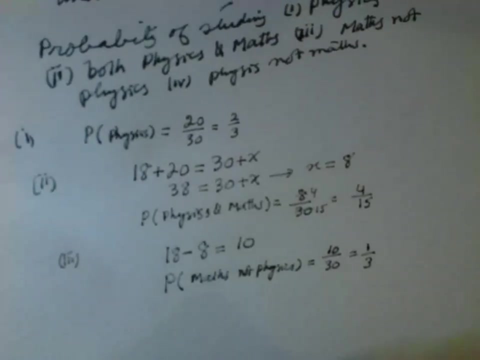 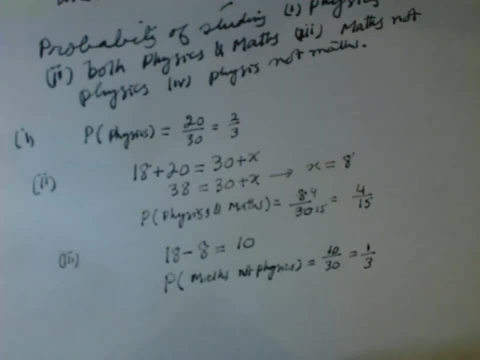 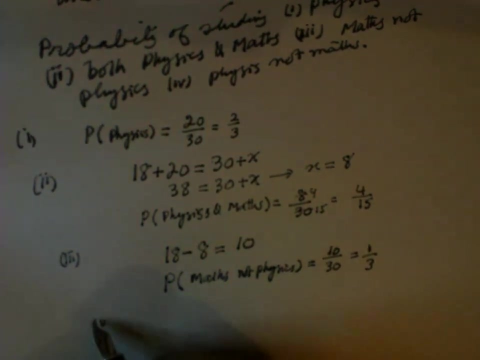 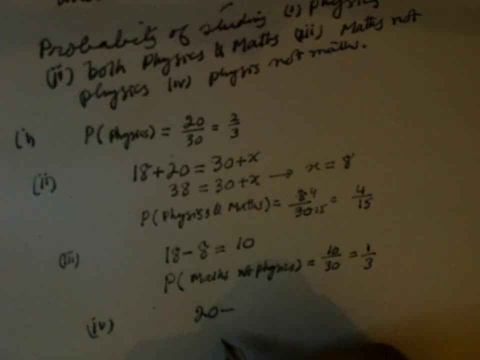 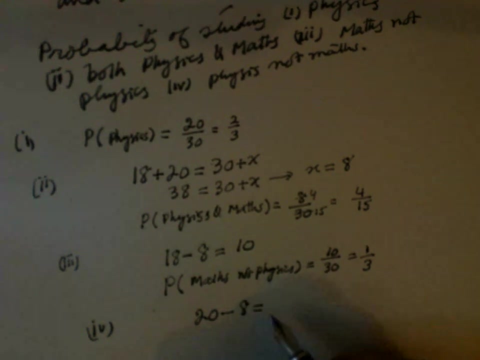 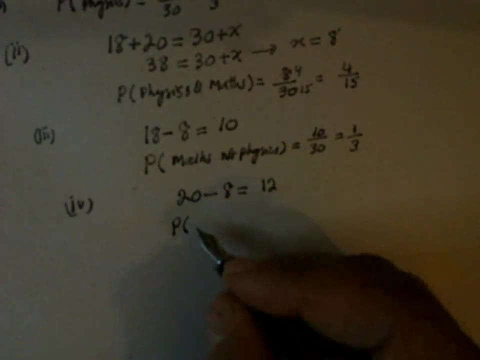 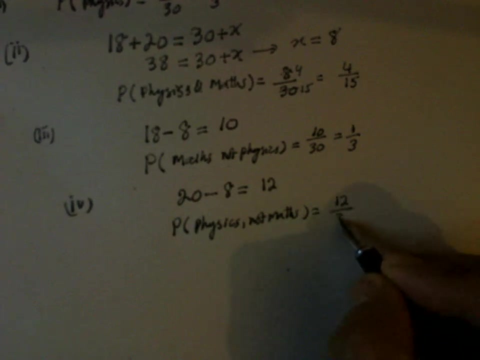 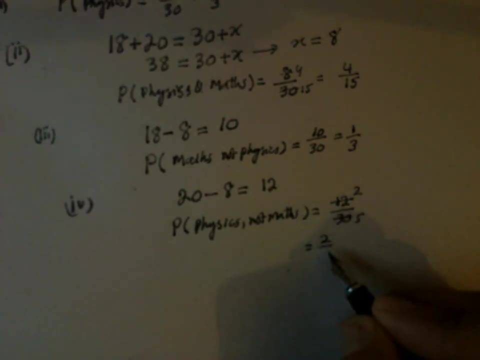 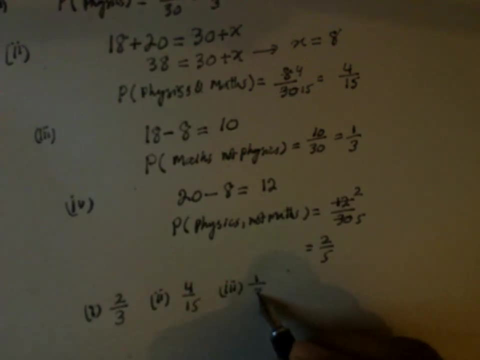 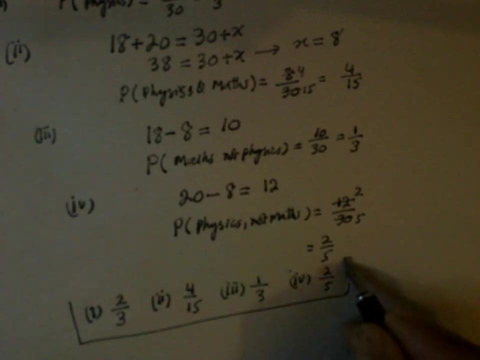 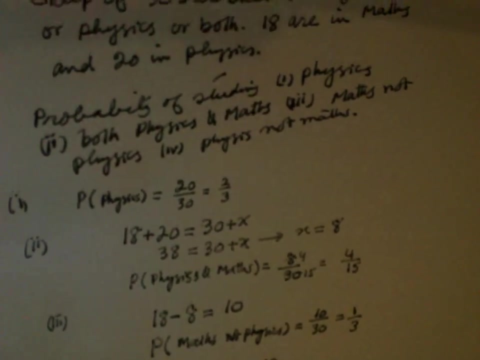